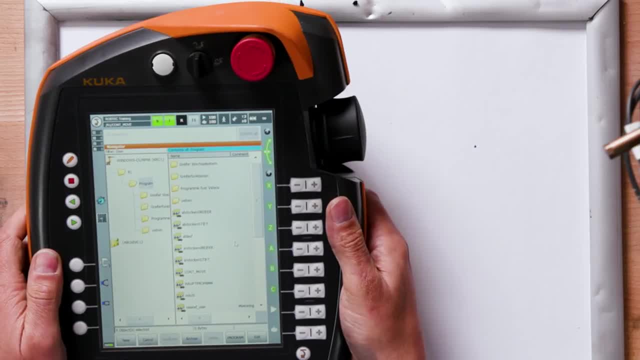 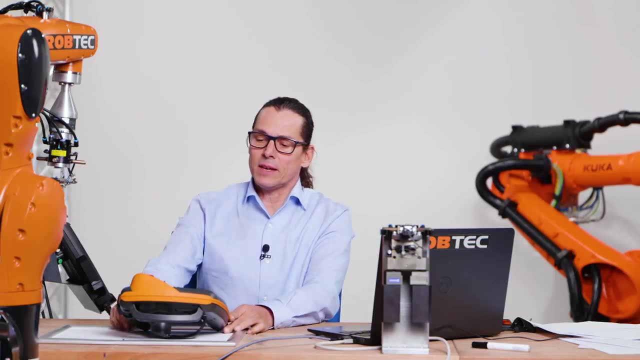 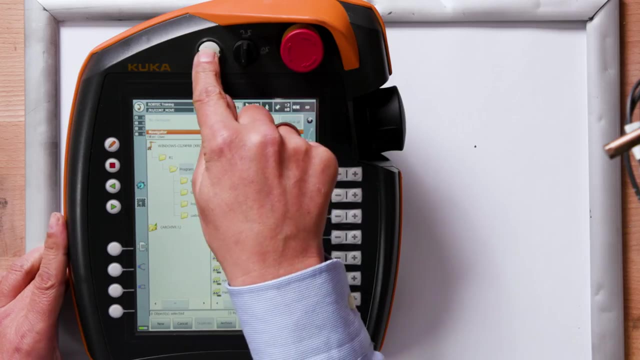 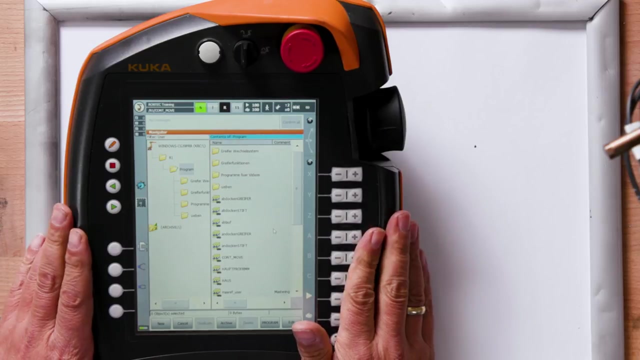 you see in the front that the green signs for movement. it's enabled, Okay. Okay, let's go to the front. First button I will show you is that one. If you push that button, you have 30 seconds that you can disconnect your smart pad. 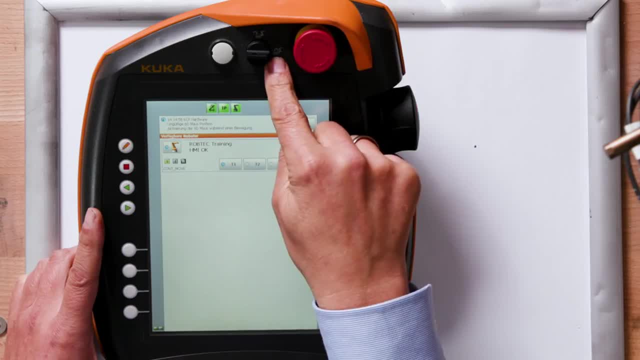 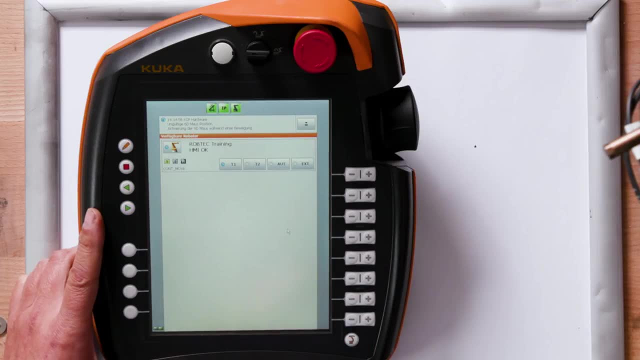 The second switch here is the operation mode switch. I enable that, and then I can choose Test 1,, which means manual mode, Test 2,, which means manual mode, Test 3,, which means manual mode, Test 4,, which means manual mode. 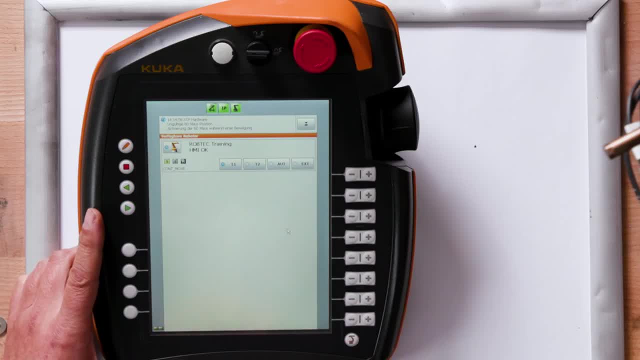 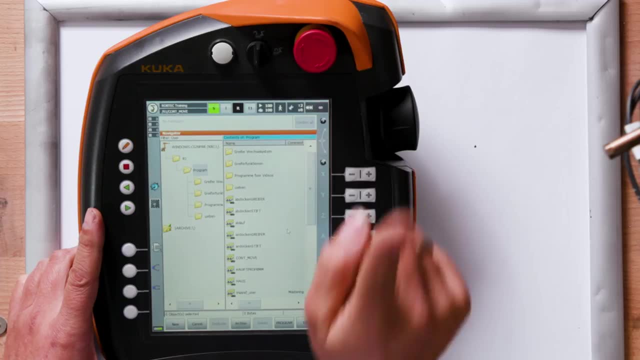 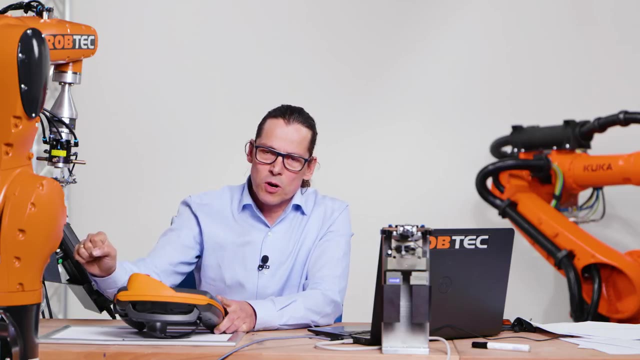 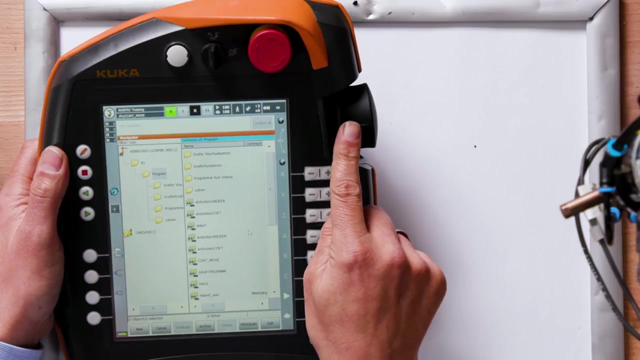 manual mode in full automatic speed. then we have automatic mode and external mode. I explain you that in further videos we go back. here is an emergency stop. when you push that button, the robot and the whole environment has to stop where the robot works. and here is a 6D mouse. 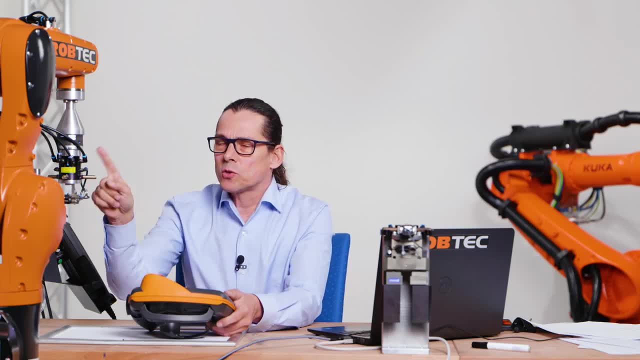 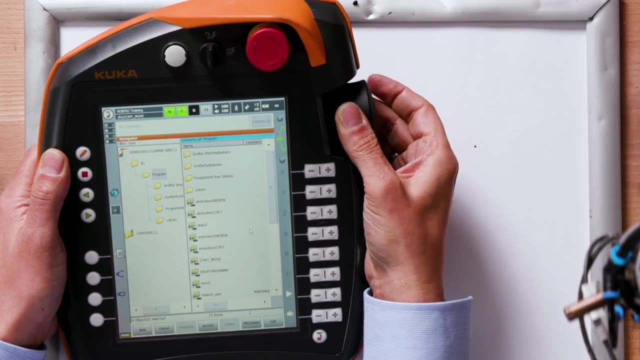 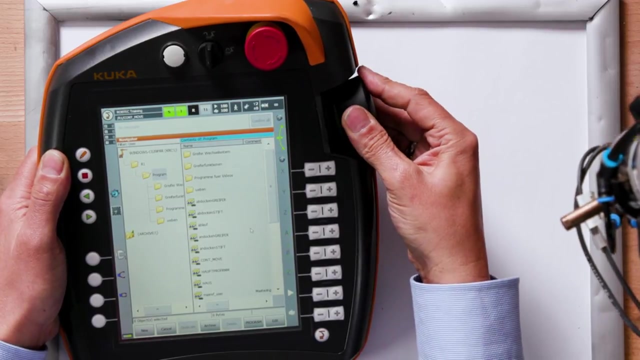 you can use this mouse to control the robot. that's for experts. please have a try. what happens? that if I push that button, the robot will move. if I pull, it moves in that direction. if I push it to here, it exactly moves like the robot is and I can move it up and down. and if I turn it, it's moving like 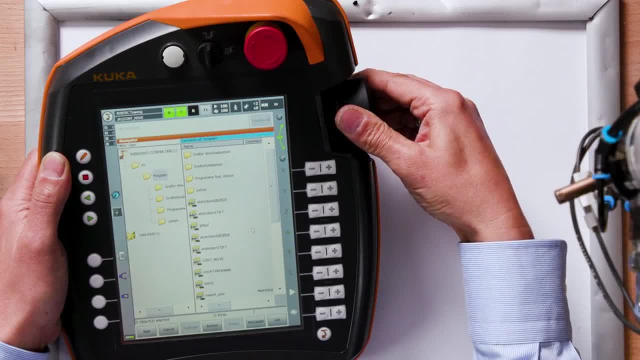 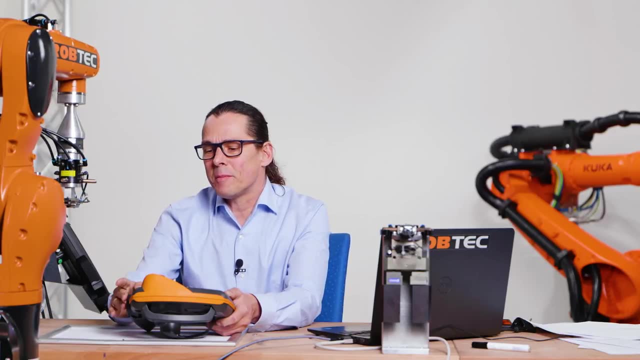 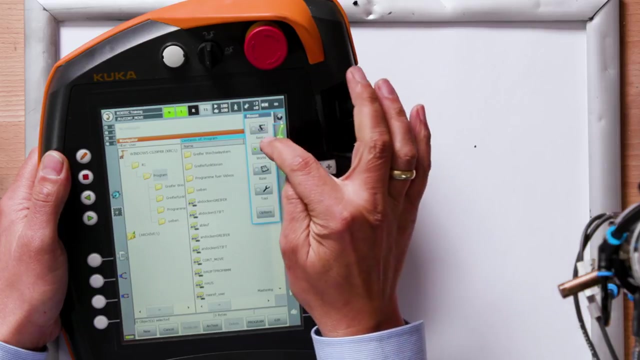 that I can make that and I can turn it like that. so if you like, try this mouse, 6D mouse. if you're a beginner I would say you should prefer that buttons. you can see this is x plus in world coordinate system. you can choose for your mouse another coordinate system then for your buttons here. 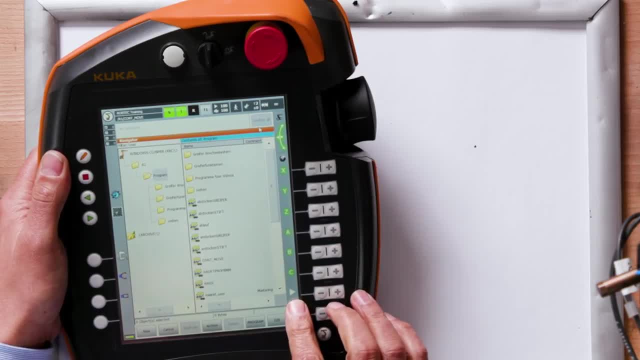 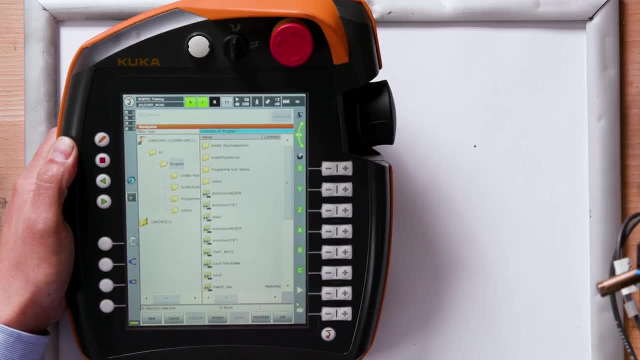 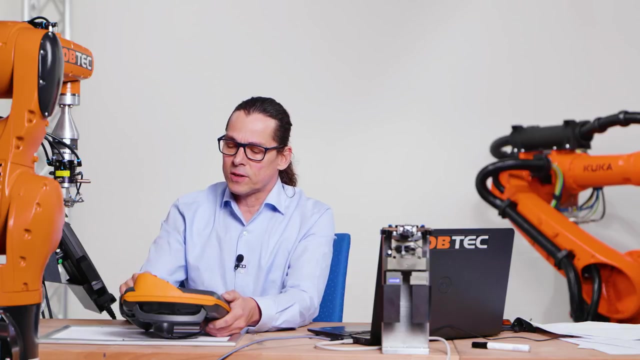 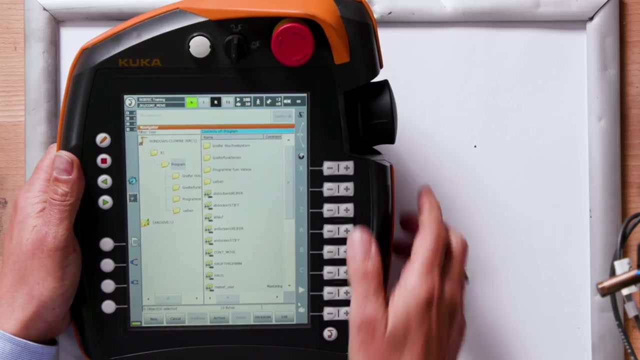 okay, x, y, set on the button. here we have the play symbol and that means we can choose the override of the program. you all, you see it here, how fast the robot moves. and uh, here we have the hand symbol, which means how fast the robot moves when I move it with the. 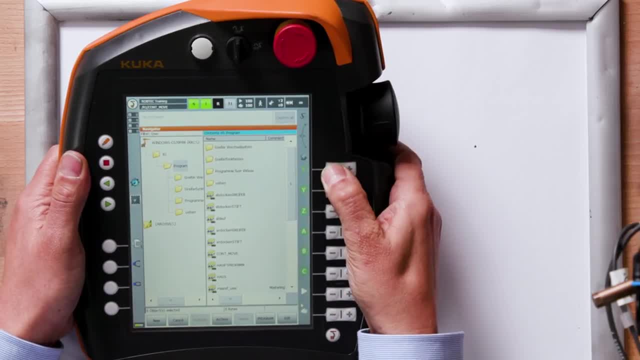 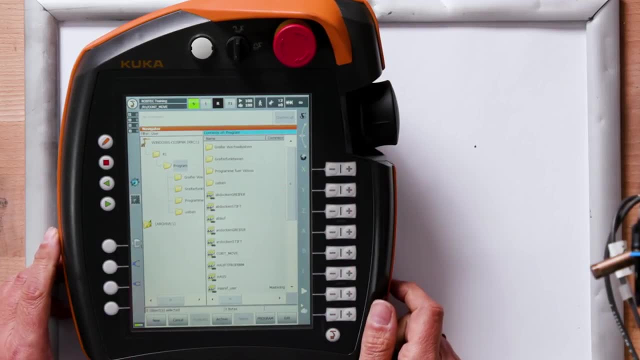 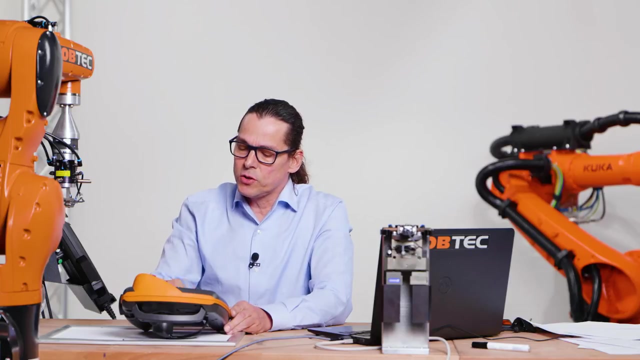 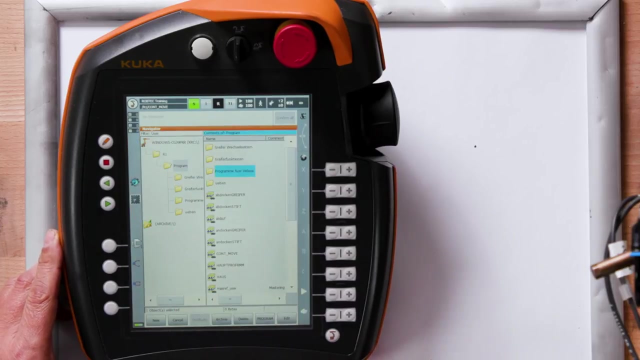 buttons or the mouse. If I choose 100% here, Robert moves faster. This is to move very accurate. I reduce the override from the hand On the bottom. here I have some menu signs I can choose. Depends on in which menu we are. We will see this. 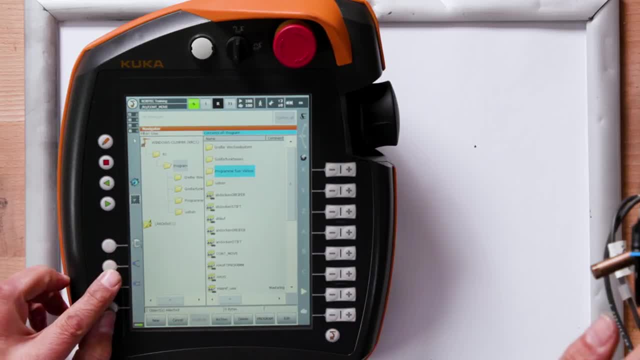 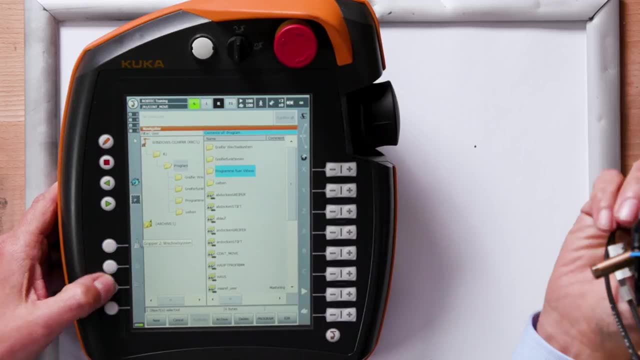 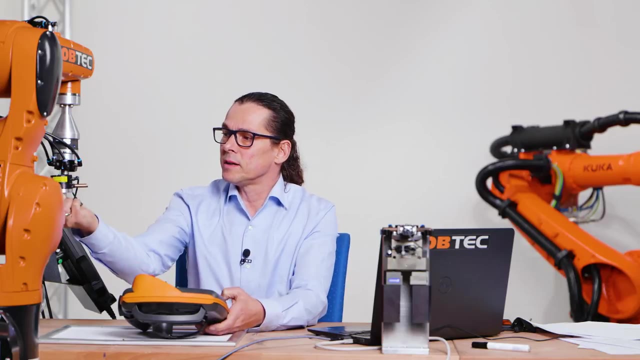 later. Here on the left I have buttons to control the gripper, for example. You can program that to your needs. We have a docking system and I can open and close the docking system to do that or open and close the gripper. Here we have. 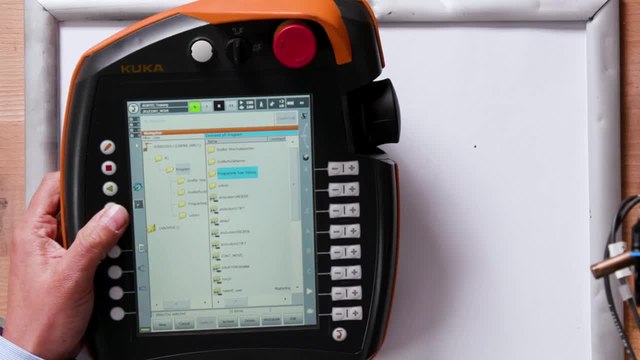 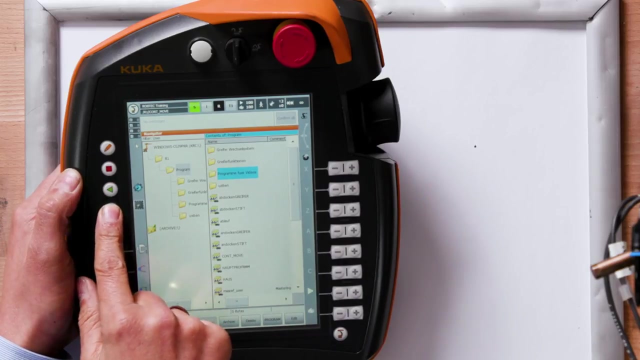 a play plus button and play minus button. Play plus means the robot moves forward the program and we also can move backwards the program. That one has more explanations. It only can move backwards that what we moved before forward. Forget it. I use the forward. 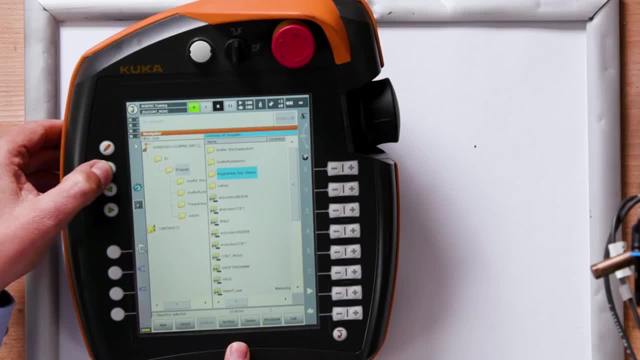 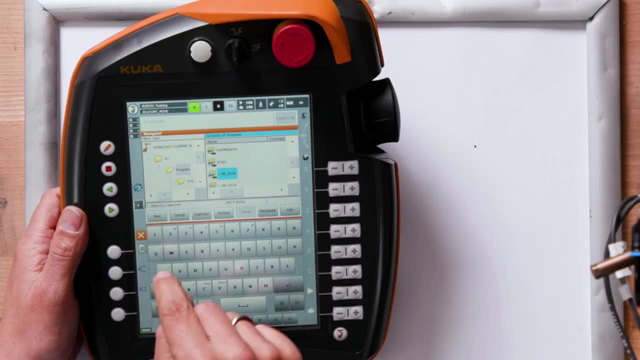 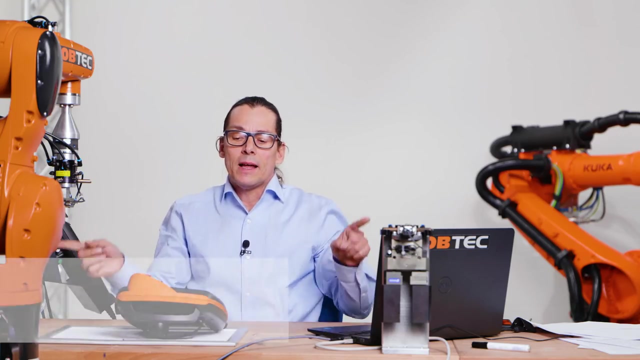 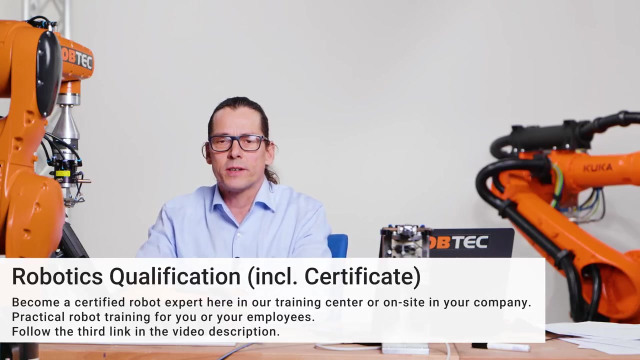 button. This is the stop button. If you start a program in automatic, you can stop the program Here and that sign means you can choose your keypad here and you can write something with that thing. Okay, let's go into the PC. I show you the same what is? 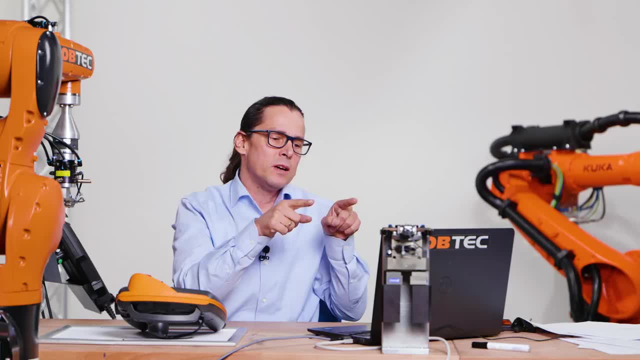 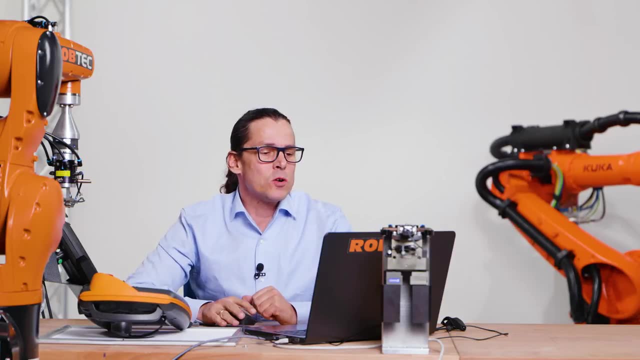 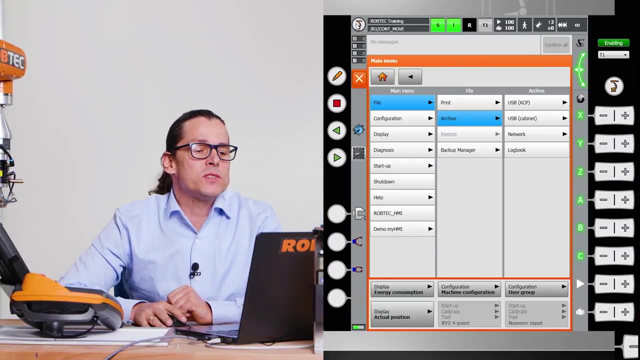 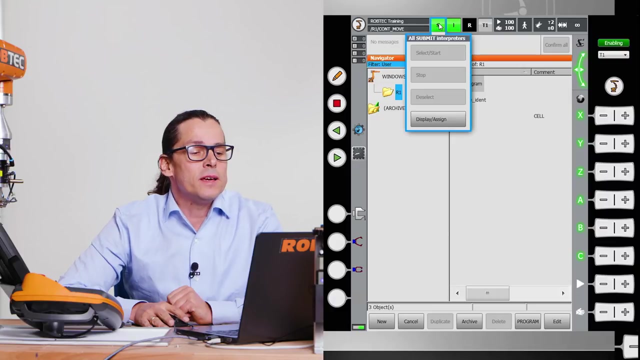 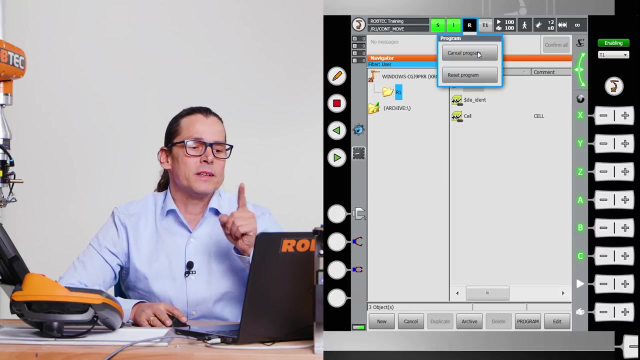 here. but for better resolution of the screen I show it here, Okay. Okay, let's look inside the touchscreen. here you see the cooker symbol, which means you can. you can open the menu there. you see the submit interpreter. I explain you in further videos. that button is to cancel and reset programs. you have to cancel a. 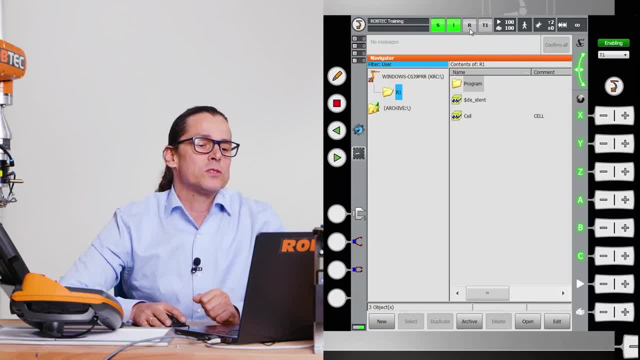 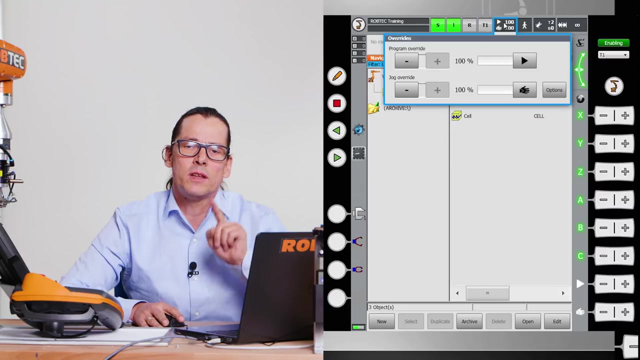 program. if you want to select a new program, so, and if it's already canceled, that button is gray, when otherwise it's black. or if a program is started, it's green. you will see this in further videos. this is the mode, the operation mode the robot has. now we are in manual mode. that means test one. here you can. 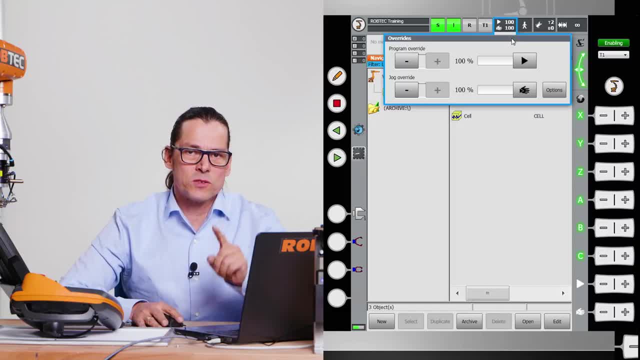 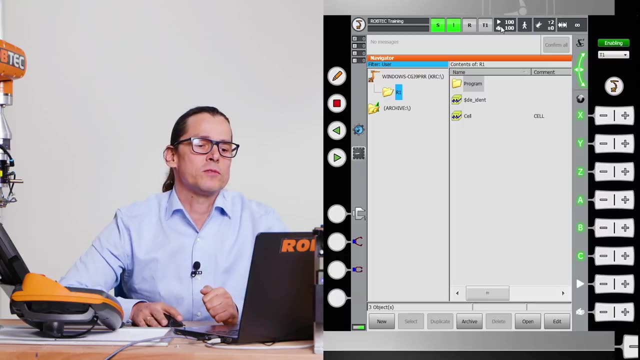 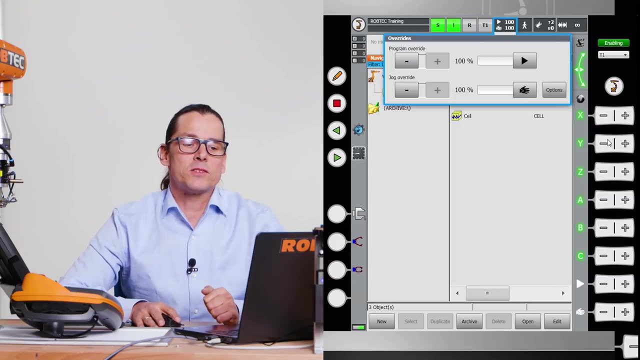 see the override. you have two overrides. one is the play override, that's the override from the program. one is to push the play button. the robot plays with that override, the program. so 100 is 100% and 50% is half of speed, and the manual override, that is. 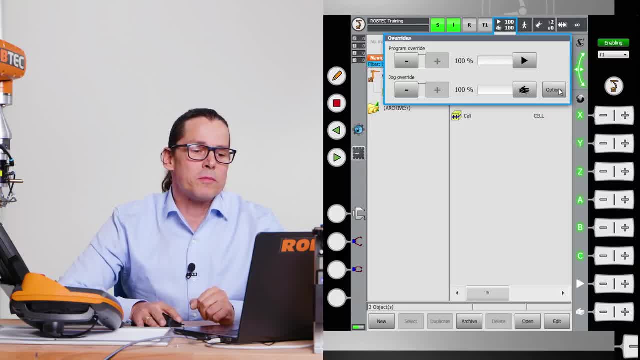 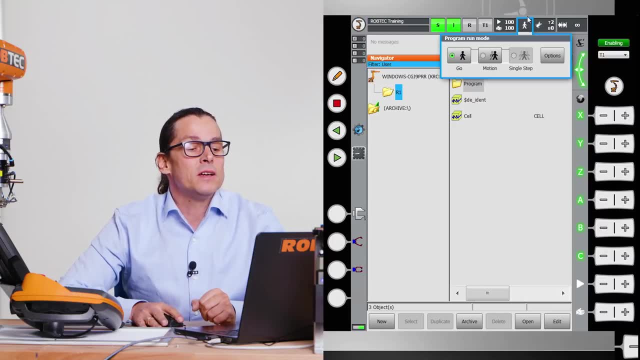 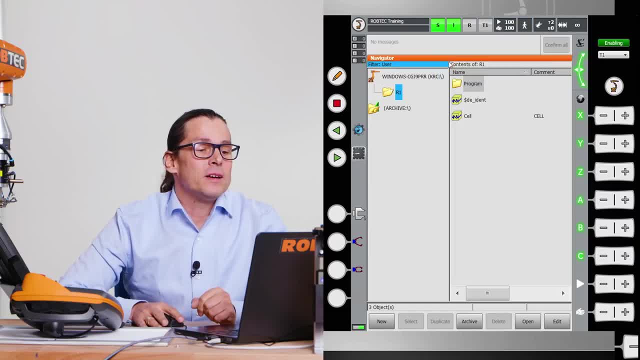 is one man walking or woman, and then the robot will continue to program as long as I push the play button when it choose the second one, then the robot stops at every movement, all that the signal stuff it will play like on, on on the man walking sign. but when I start here, Robert stops every movement and I 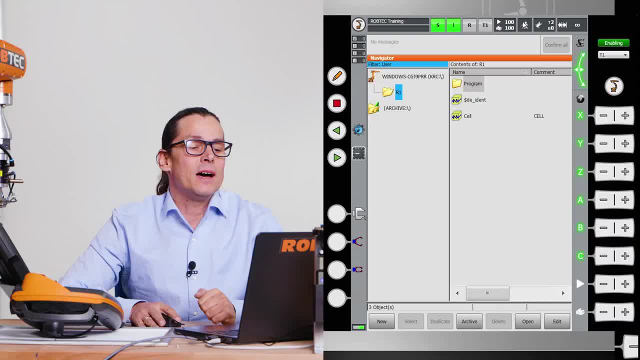 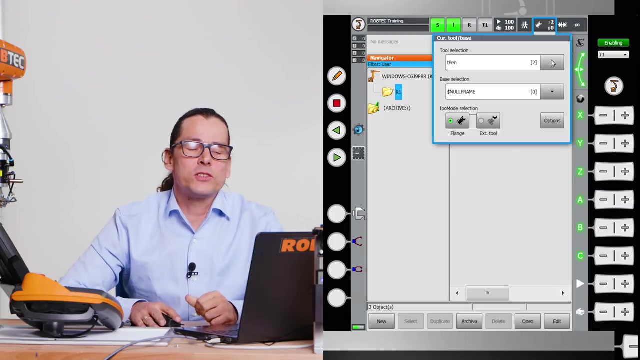 have to push the play button again. and single step movement is that? for that you have to start every single command in the program. so you can debug very well with that sign. okay, here I can choose the tool I want to use. so we have different TCP's. yeah, if you don't know what a TCP is, look at my other. 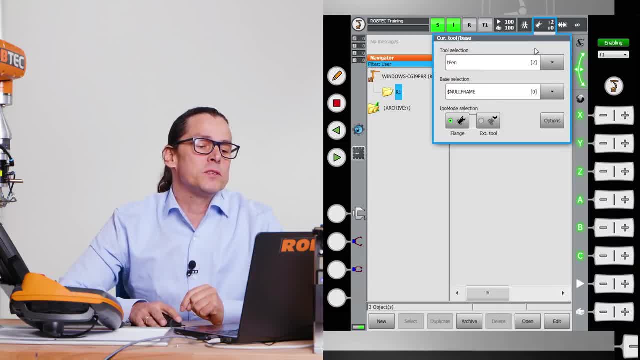 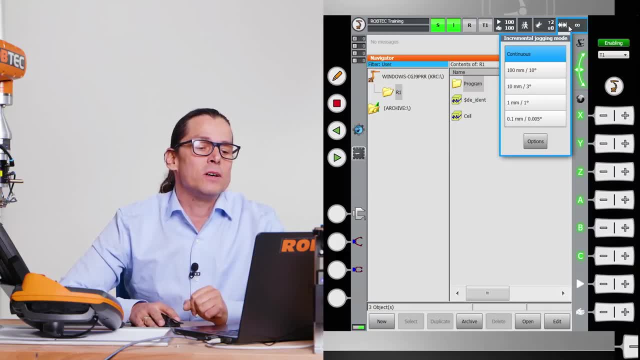 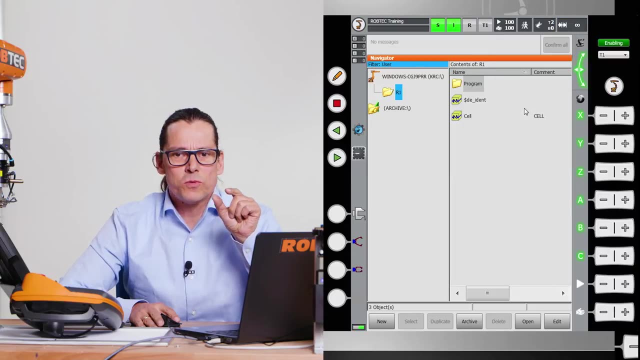 videos. with the TCP you can choose the TCP and the base and also you can say an external tool. whatever. we skip that one. this is just a. if you move very small steps, one millimeters, you can shoot that. normally you don't use this here. you can see the mouse movement is now in axis mode, so 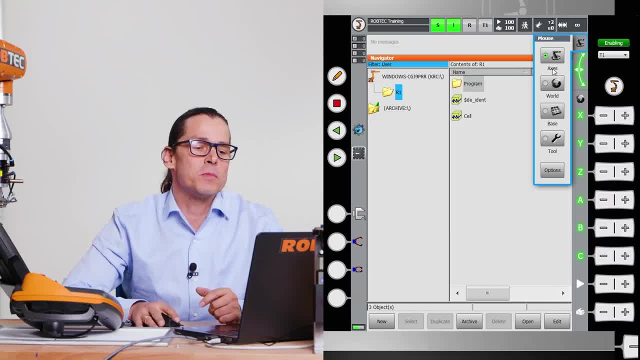 when I'm moving with the mouse on on the smart pad. it should. it is in axis mode, world mode, in base or in tool mode. you can select it here and that sign is for the buttons to move the robot it. and I have that in a different modes than the mouse here as a cooker symbol. 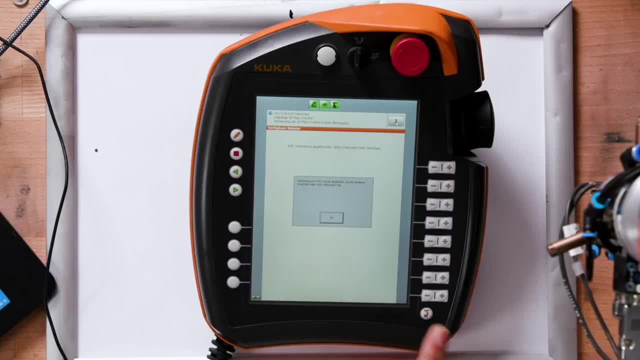 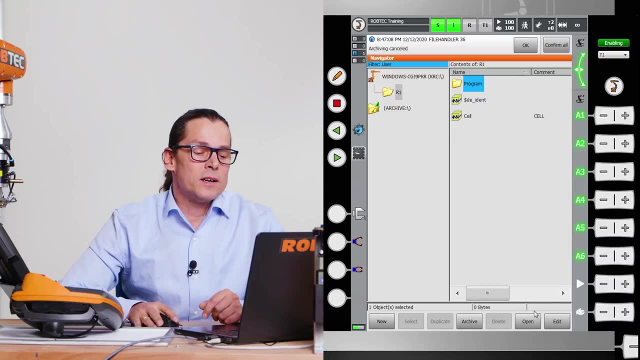 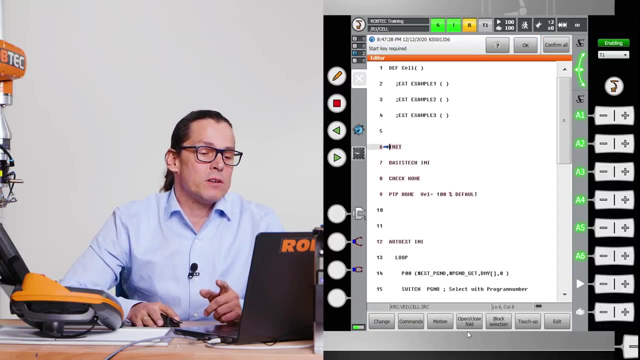 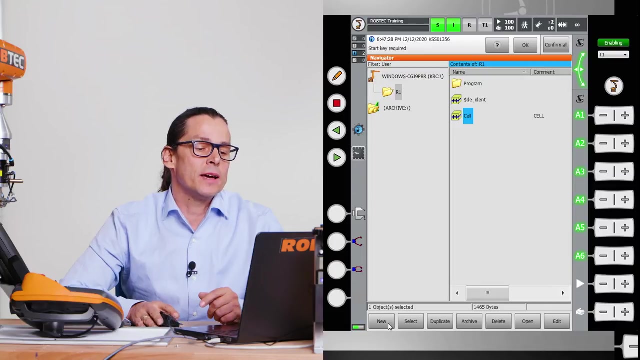 in our smart pad in real we have set on the right button here you can see individual menu inside the touchscreen. it changes whatever you have selected. it changes what you can do here. I cancel the program and you see there are different things you can choose. good, here are the. 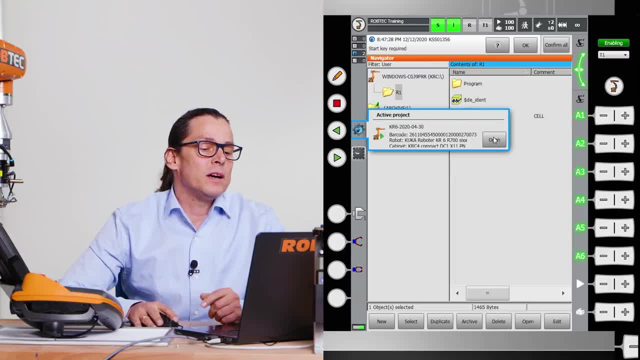 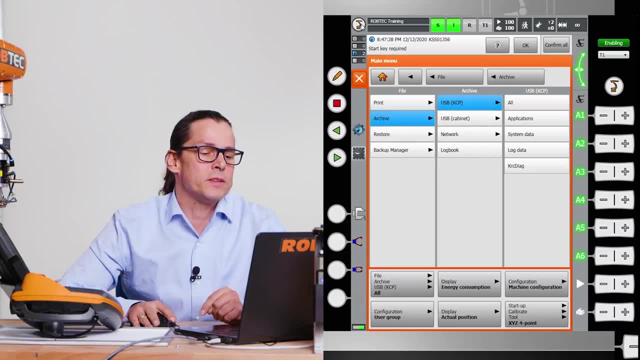 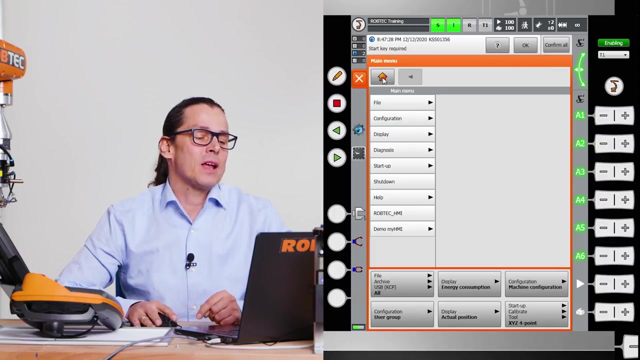 symbols for the buttons here, and here is your project for work visual. I will show you that in a further video. okay, let's go into the main menu. when I choose that cooker symbol here, cooker symbol here or here, I can go into the main menu by clicking the house button from there. we have our most important points here on. 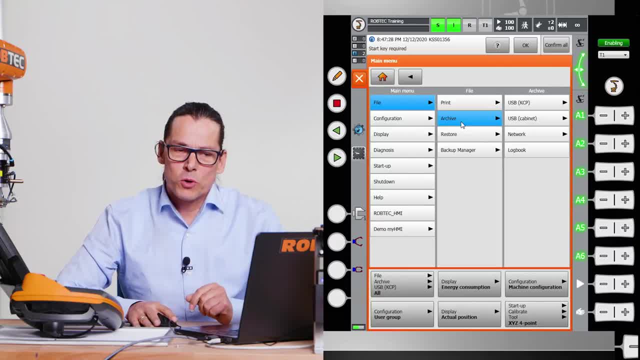 the left side if you choose file. important thing is to to make them back up from your robot. if you use the USB on your car CP, which means the smart pad or the USB on the cabinet, that one is the controller. you have USB stick, USB ports there and you take your USB stick and you make an. 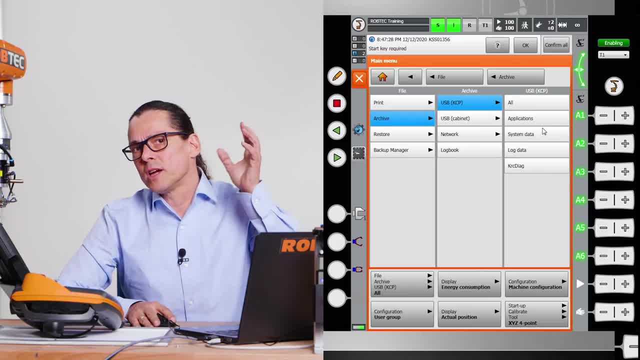 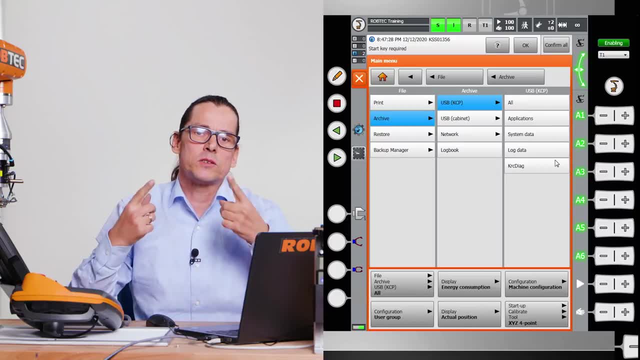 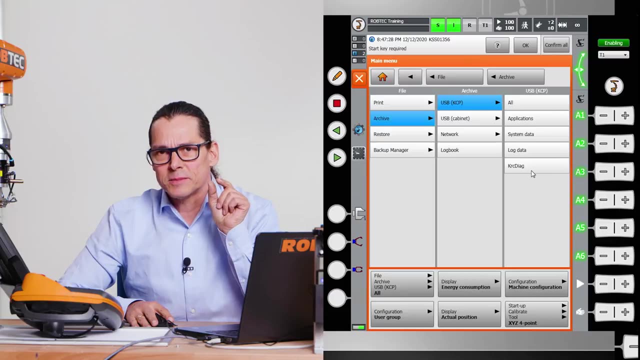 backup. by clicking all, you have a backup of all which is in the controller. if you have some problems with your robot and you need the cooker support, you can save a diagnostic file on your USB and send it to cooker that they can help you better. if you have a hardware issues, that is the car LC. 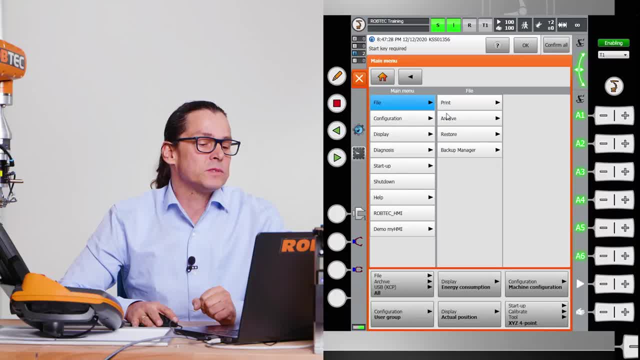 Diag or log data. yeah, forget about the rest. you need that one and to restore your backup, you can choose that. choose where, from where your USB stick sticks and you can restore your backup again. if you have any fault, let's go to the next button here. this configuration: 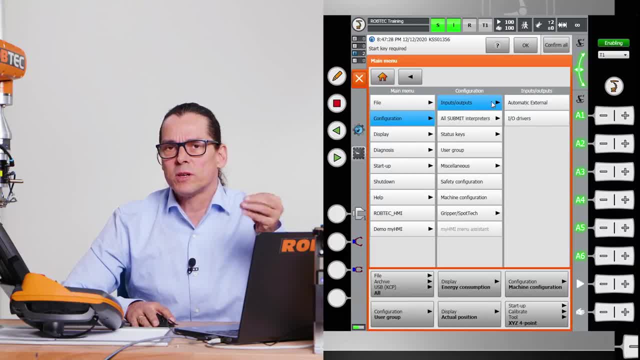 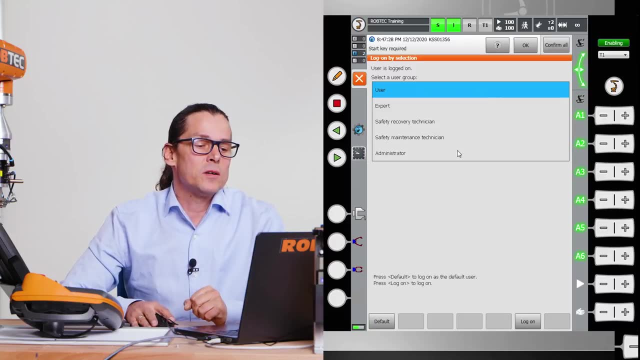 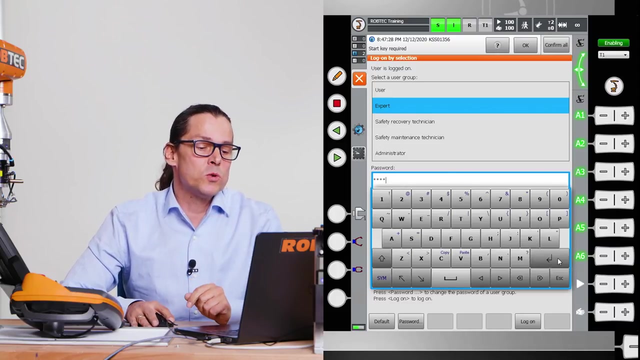 you can configure your probe of your robot, for example the inputs and outputs. you can change the names, you can say your automatic addresses, you can change your starters keys, that once you program here, you can change the user group. we will change now to cooker, to to expert file. 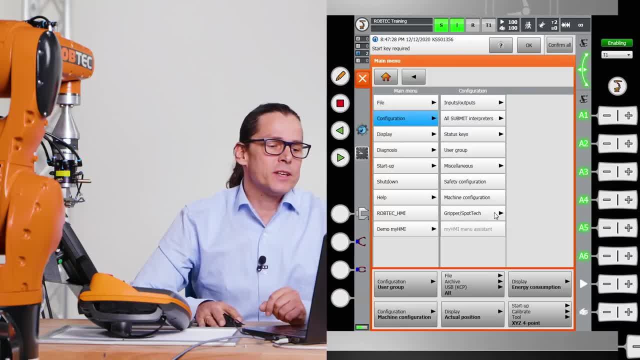 computer we can see what typically the user group or if you have any associated with Hoover perfectly this history. you can please constantly watching the reatittutorial November. by clicking the next menu sections. the configuration opens a sub menu where you can change the correlation of your inputs and 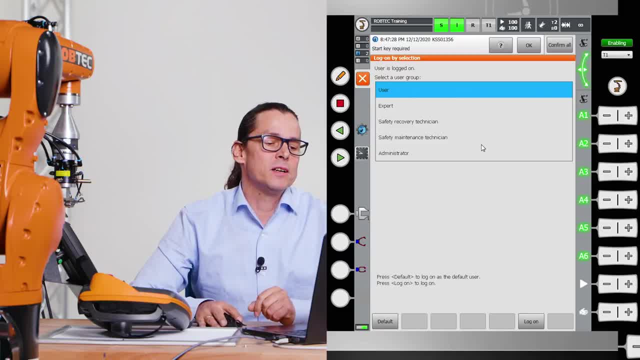 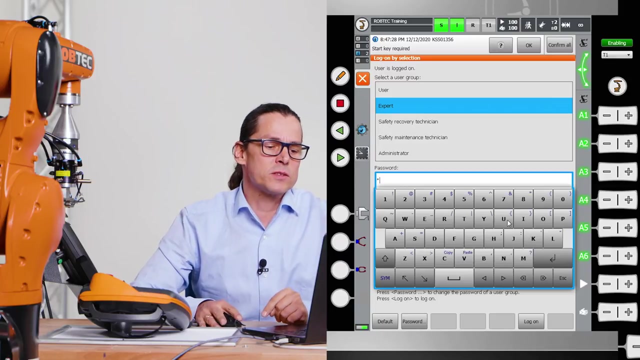 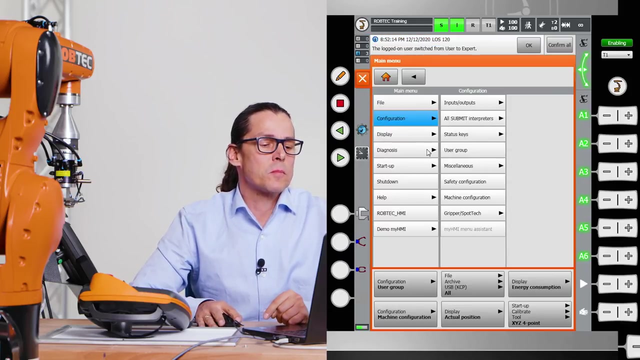 outputs something. interpret so statue keys, which means that keys. here you can configure what you want to see. here you can change the user group, which means a, your user. you can start and stop programs. you can teach positions if it's allowed, but if you want to see more, you have to change to expert, standard experts. security word is KUKA from now. 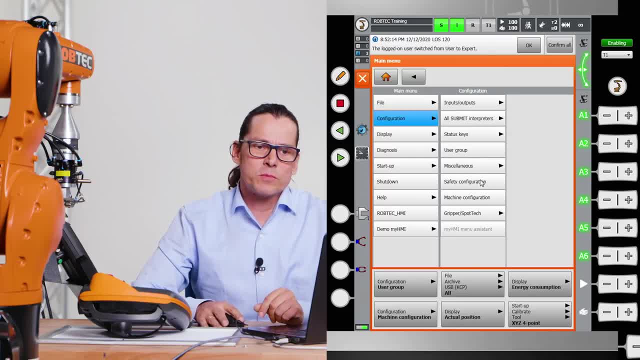 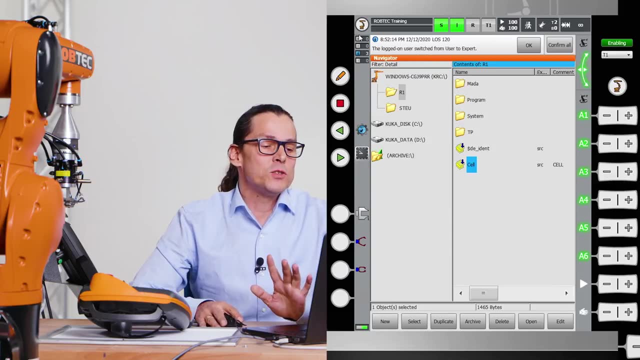 it looks a bit different and have me more possibilities to control the robot, the safe configuration you shouldn't touch and all the other things. here you have grippers. spot that tech. you can change some other things. please don't touch it if you don't know what you do. 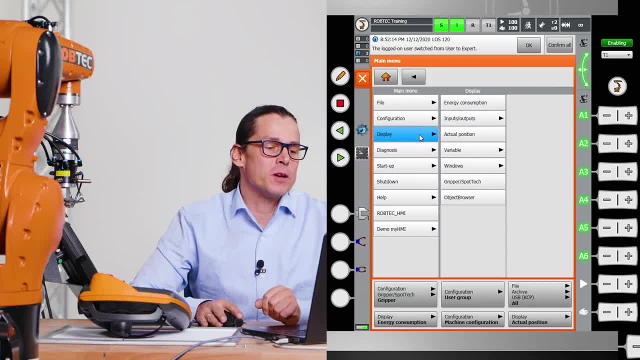 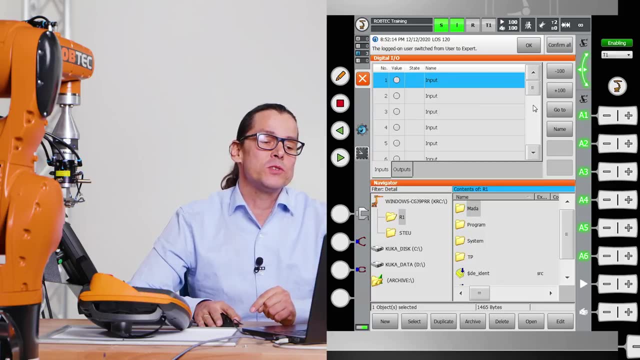 anyways, the configuration tab is for programmers. okay, let's see what happens in this play. in this play, you can see such important things like how much energy the robot needs. I think don't this, don't care, but sometimes you need to see your digital in or outputs to analyze what is. 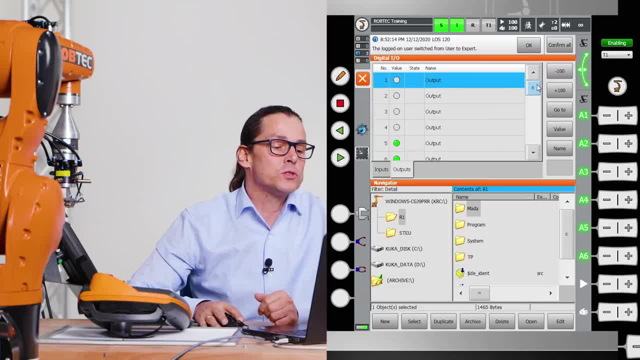 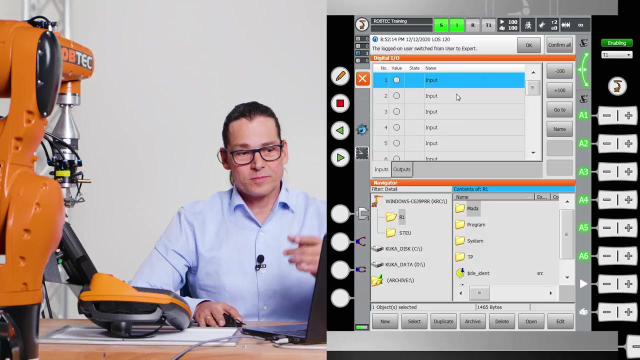 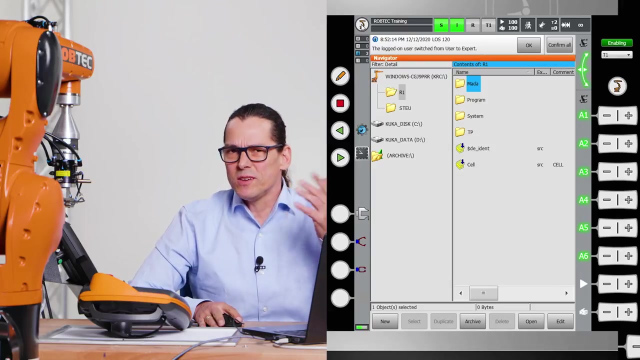 maybe the robot waiting for and you can choose here outputs and you see if an output is one, you see it here because it's green, otherwise it's gray. gray means zero, one is green and the input you can see here is no input. you should name the inputs here by clicking that button to see what really. 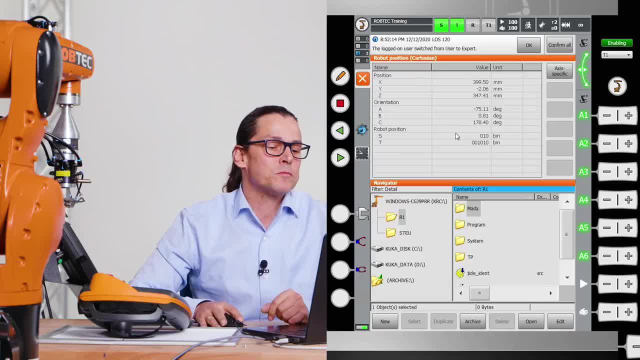 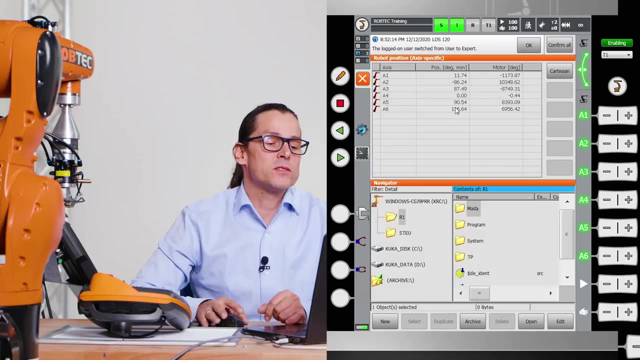 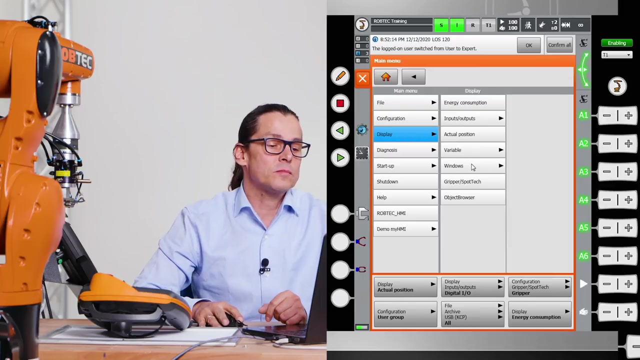 happens, for example, gripper open, gripper close. okay, that's a display, you can see your actual position. this is maybe interesting if it changed to axis. you can see how many degrees the axes are and software limits, which you can check. that here in display, actual positions, you can see your. 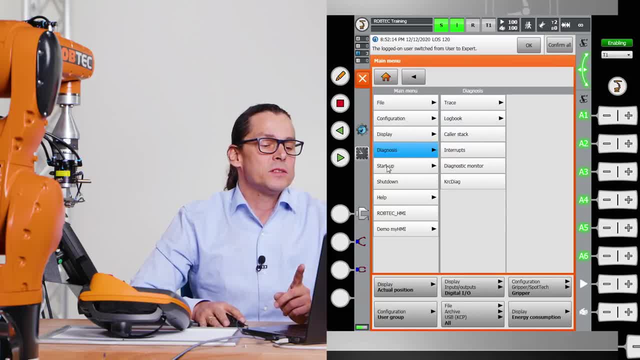 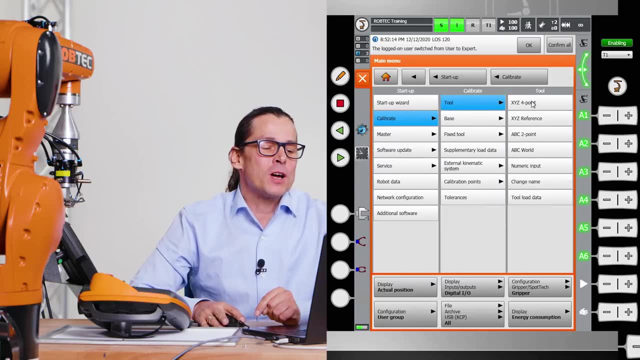 variables, uh, some other stuff, diagnosis- I think you don't need this, so, but startup, startup. we have something, so we need to. I show you that in in the robot channel here: how to calibrate, uh, the tool. yeah, you saw that in the video. I just showed you how, the way to calibrate the tool. so how to calibrate. 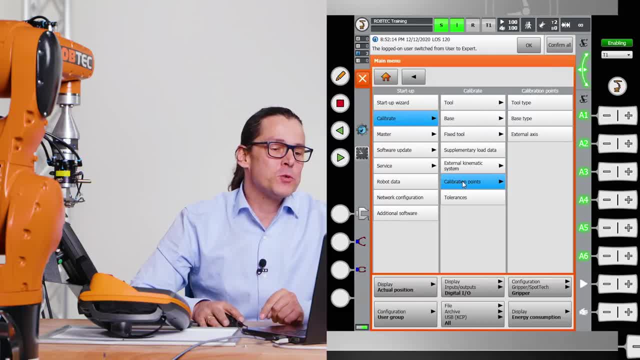 you saw that in the video. I just showed you how to calibrate the tool. yeah, you saw that in the video video before the base. you will see it in a video here: a fixed tool, calibration points, etc, etc. how to master the robot. the robot has to be mastered. I will show. 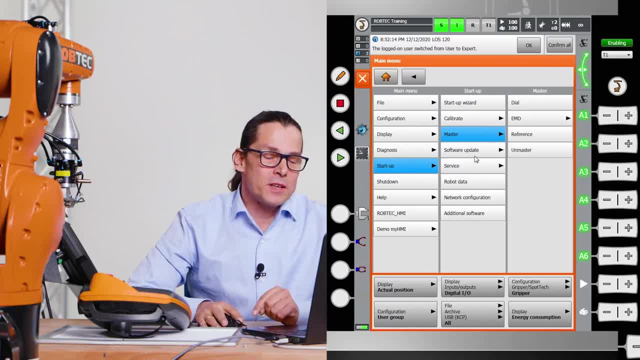 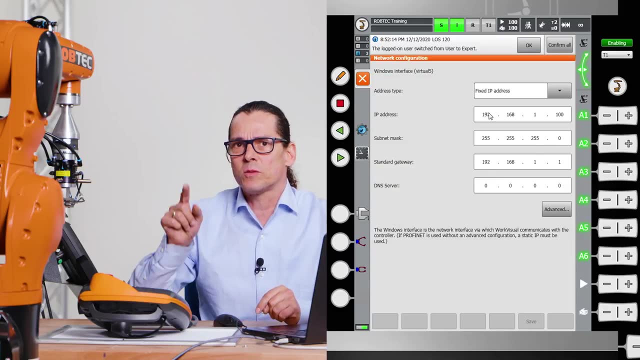 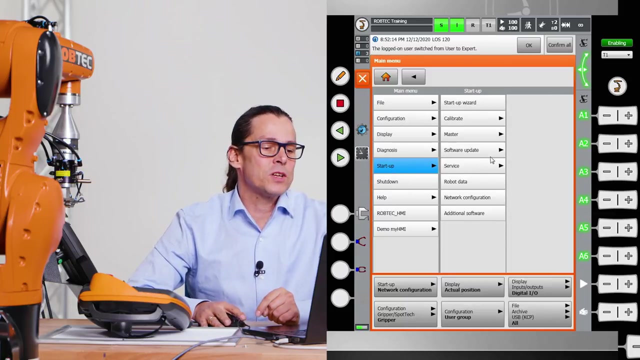 that how to do this. you can update your software, your software. please be careful with that. and one of the most important things is a network configuration. if you start programming your robot, you need to know your network address. you can check this here. good, let's go to the 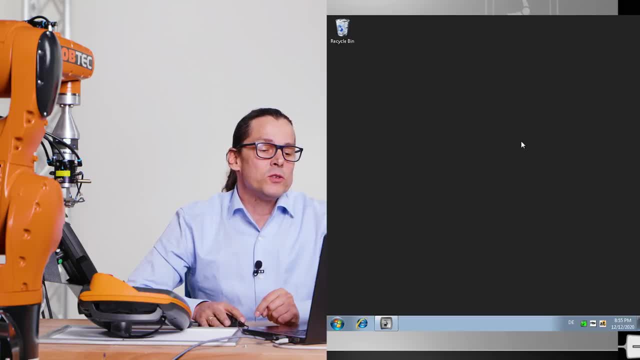 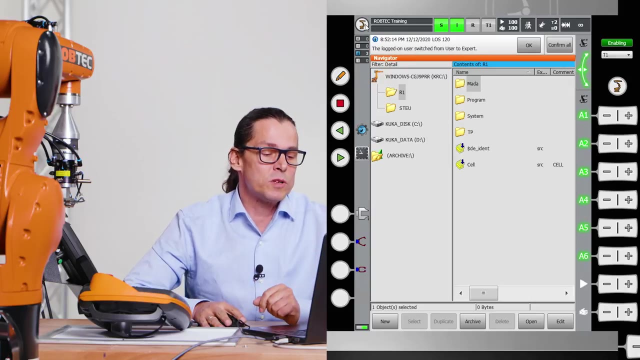 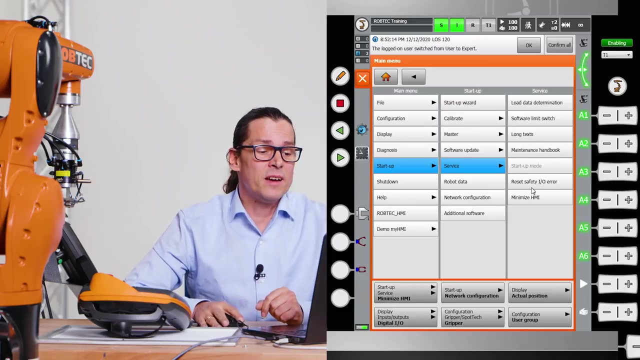 service button here. that is one thing you can use to go back to your windows. sometimes you want to install maybe some game. so no, please don't install games, but here is normal windows. so sometimes we need to go back to windows and yeah, for diagnostics or something like that. 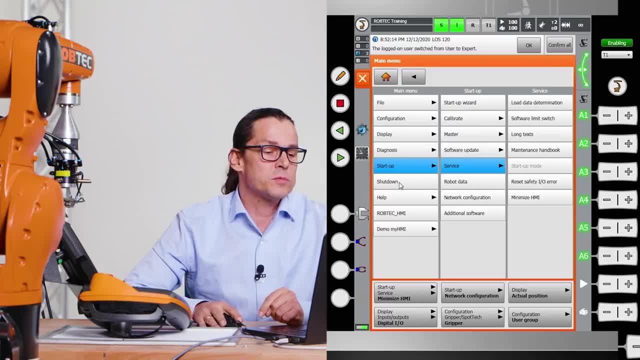 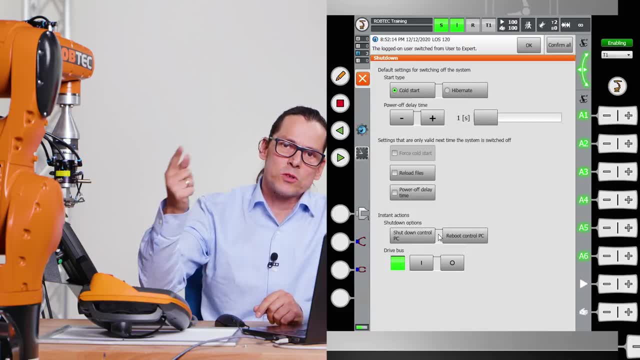 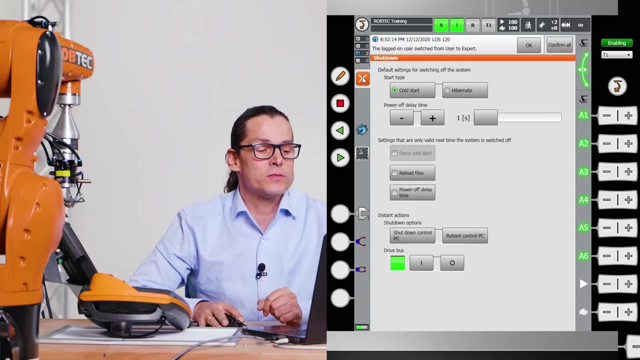 you can do it here, only available if you are an expert. okay, shut down is to restart the robot controller. you can select if you want to reboot the PC, if you want to reload files, if you change some configurations files. just ensure that you have selected this button. yeah, windows is on this. 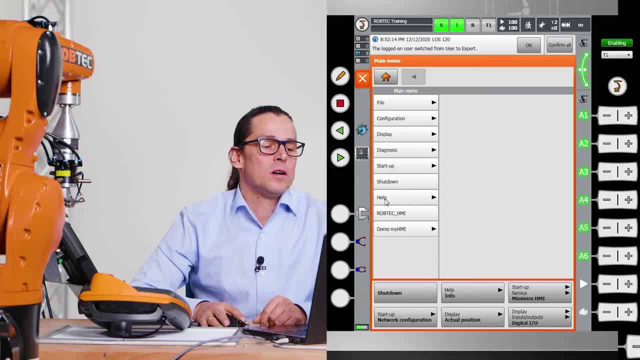 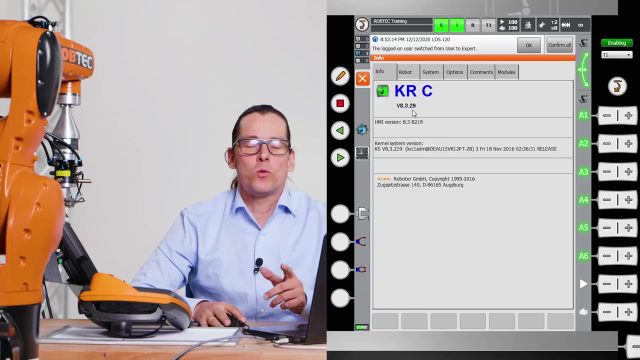 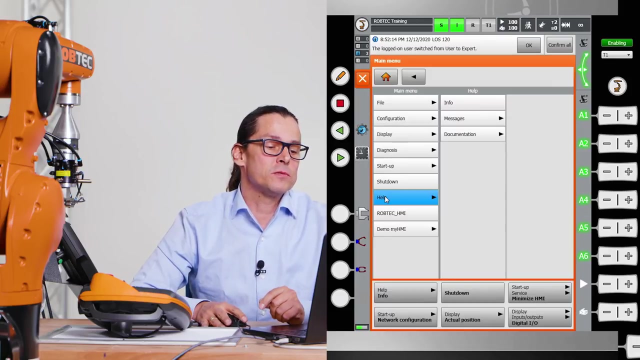 robot. so sometimes you have to reboot. okay, and we have a last button here. you see some more I programmed. forget it, as the last one is the help button. in the info tab you will see which software on the robot runs, which robot. you have the system and all that stuff for informations and another thing. 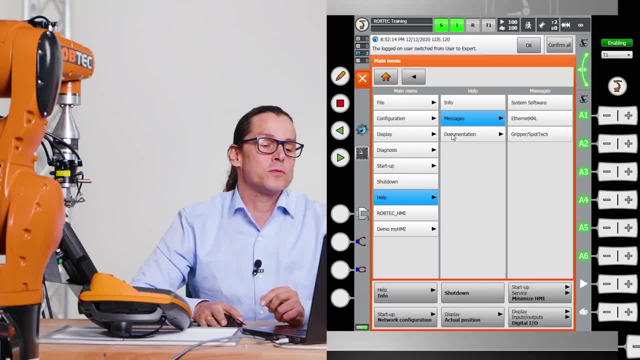 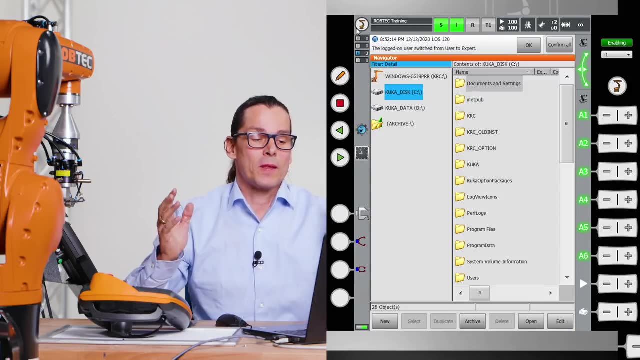 is the messages from system software and the documentation. there's a complete documentation how to program the robots. the manuals are inside there almost, and then you can see here the software. you can look to that. Yes, that's the main menu and quick guide through the smart.